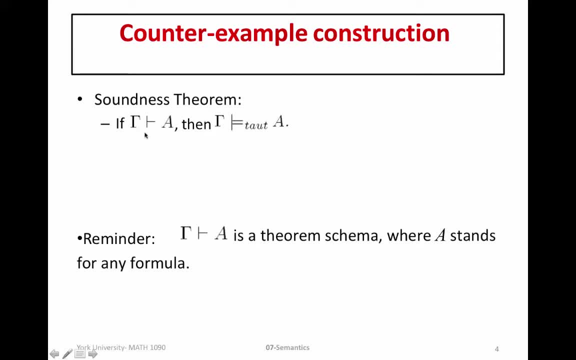 And in the case that gamma is empty, for example, then we know that if a is an absolute theorem, then a is a tautology, Or essentially, every absolute theorem is a tautology is what the soundness theorem says. So those are a number of different ways to think about what the soundness theorem says And those are all helpful in the construction of our logic to ensure that it is in fact sound, that everything it proves is in fact true. So it does. 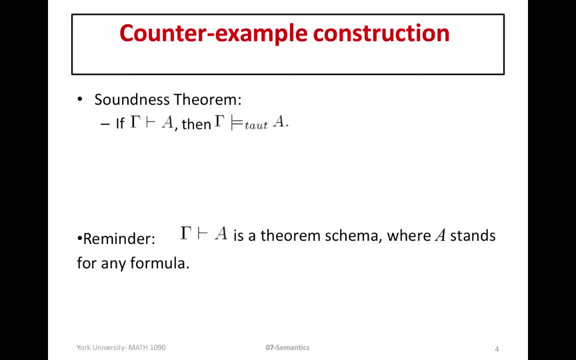 doesn't prove anything. that isn't true, which is really important. But, as I mentioned before in the previous video, we're actually going to use soundness to help us prove fallacies, So, in particular, to disprove particular well formed form or to justify why a particular well formed form is not a relative or an absolute theorem. You may recall. 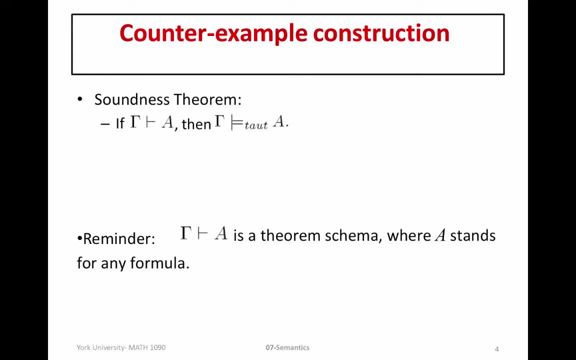 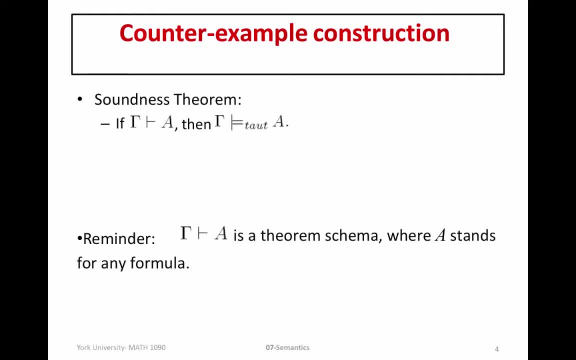 such a statement is actually: if not Q then not P. So, in particular, the contrapositive of the soundness theorem says: if gamma does not tautologically imply A, then gamma does not prove A. So to show that gamma does not prove A, it is enough to show that gamma does not tautologically imply A. Now recall, in particular, remember that gamma prove A is a theorem schema where A stands for any formula. So in particular, recall, 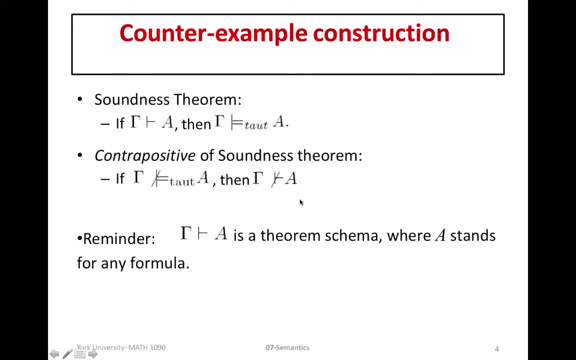 that in order to show this, so to apply the contrapositive of soundness. if we're trying to disprove a statement like this, a counterexample actually comes from this assumption here. So to show that A is not a theorem, we need to show that gamma does not tautologically imply A, But recall that this was also a schema. And so in order to show that this was not fact, 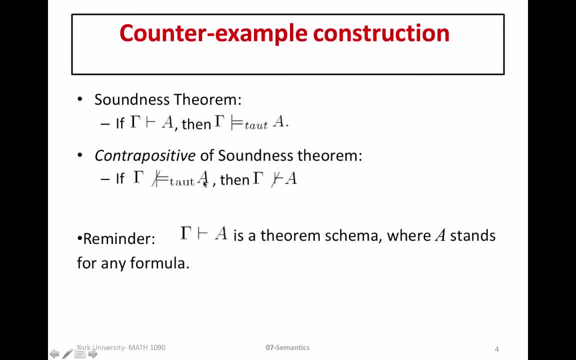 we had to find an example of A, an example of the hypotheses in gamma, and then justify this statement by finding a state which satisfies all of the well-formed formula we have in gamma but makes the example for A that we have false. So remember that we had to actually come up with examples for all of the well-formed formula within the schema. 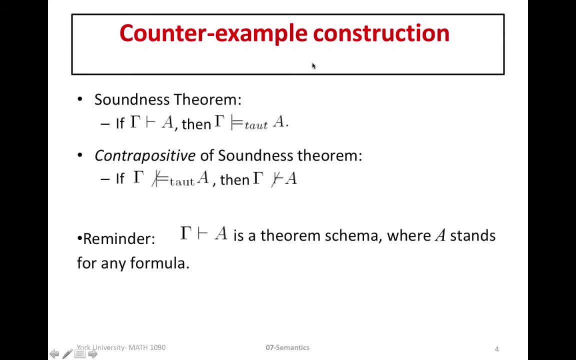 statements And that is where our counterexample comes from. So, for example, in order to show that A is not provable from gamma or is not a theorem, then we need to find- so we can, we need to find, or we can find a specific formula for A and specific examples within our hypotheses, gamma, and then some state that satisfies all of those hypotheses but makes A false. So essentially to 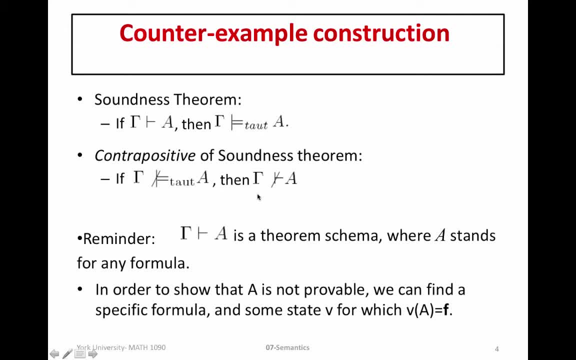 disprove any theorem, we find an example, a counterexample, and we justify this using our truth table, arguments which are much easier right. So that is what is meant by a counterexample construction within our logic here. So, to disprove a theorem, we find examples of. 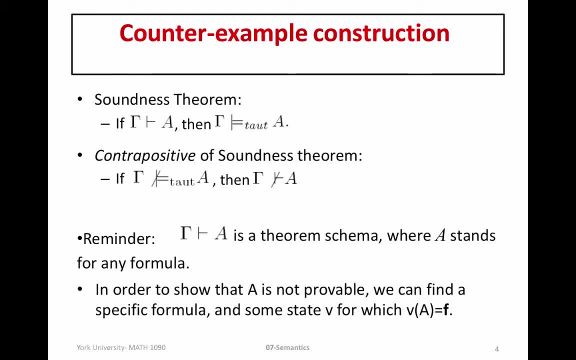 the well-formed formula we're trying to disprove and examples of the hypotheses and then find a particular state which satisfies the hypotheses but makes the conclusion false. Okay, so that ends our study of soundness theorem. here for the video, and we'll look at particular applications.